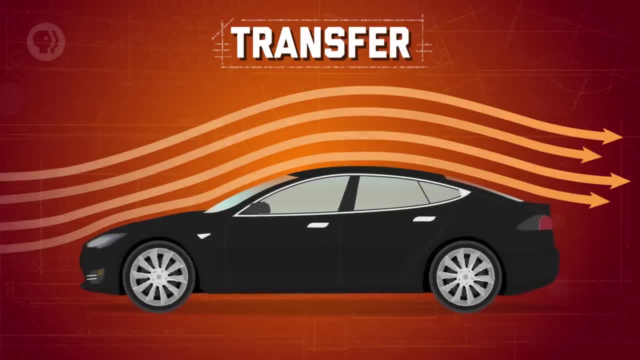 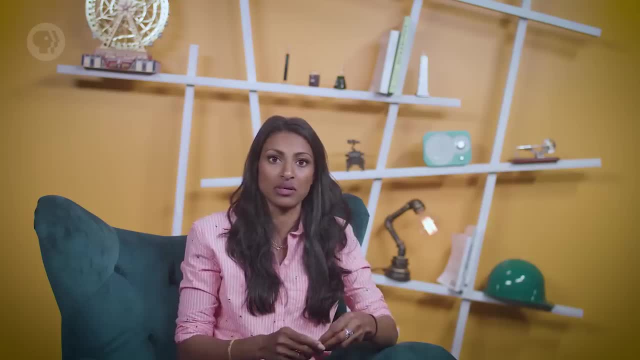 You know what transfer is right When something moves. When something moves or is moved from one place to another, There can be a transfer of momentum or a transfer of heat, maybe even mass. But if we're looking at moving fluids, then we'll often have a transfer of momentum which can be better understood with the help of fluid mechanics. 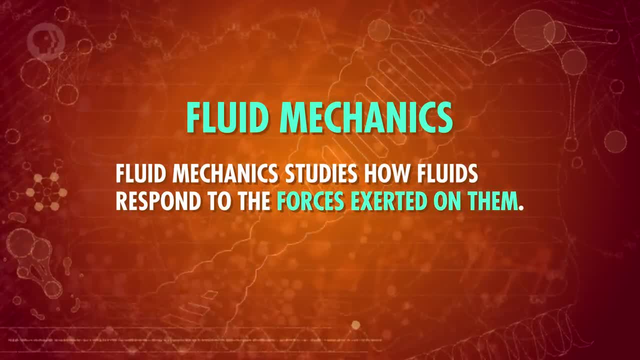 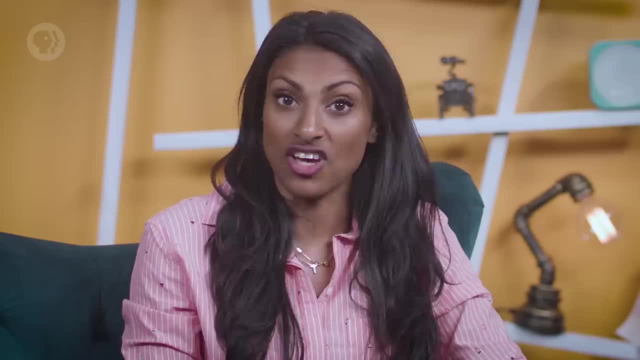 Fluid mechanics studies how fluids respond to the forces exerted on them. So how exactly do fluids move, and how does a particle, or anything for that matter, move within a fluid? To answer these questions, we need to know about stress, strain and viscosity. 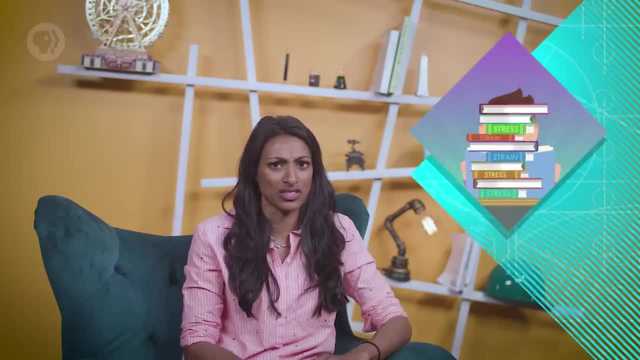 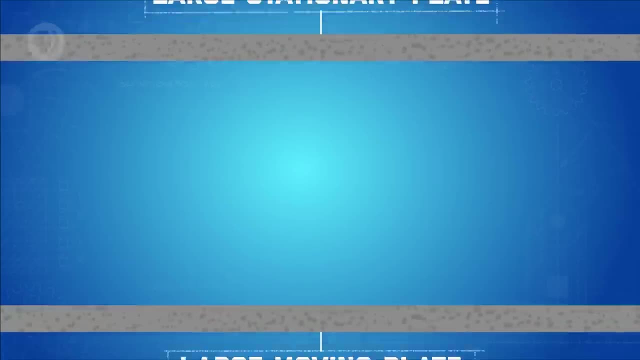 Now, if you've been a student of physics for any amount of time, I'm sure you're familiar with stress and strain in the colloquial sense, especially around exam time. But here, of course, they mean something completely different. Suppose we have a fluid between two flat plates. 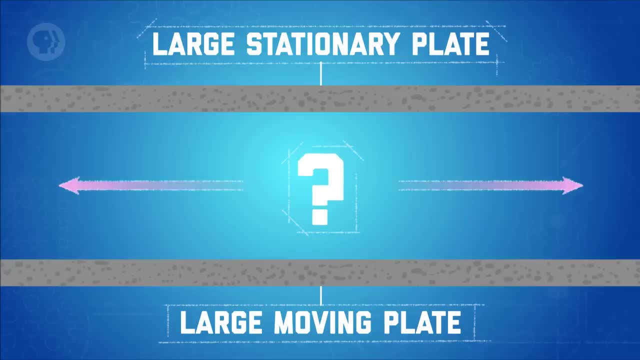 If we were to move the bottom plate, what would happen to the fluid? How would it move? Well, at the top and bottom, where the fluid is in contact with the surface, the individual particles of the fluid will go through something called the no-slip condition. 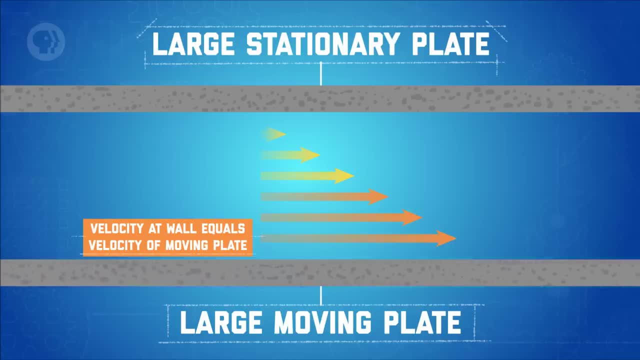 In the no-slip condition, a fluid in motion will come to a complete stop at a solid surface And assume a zero velocity relative to the surface. Basically, the particles of the fluid that are touching the solid will stick to its surface, meaning that they won't slip. 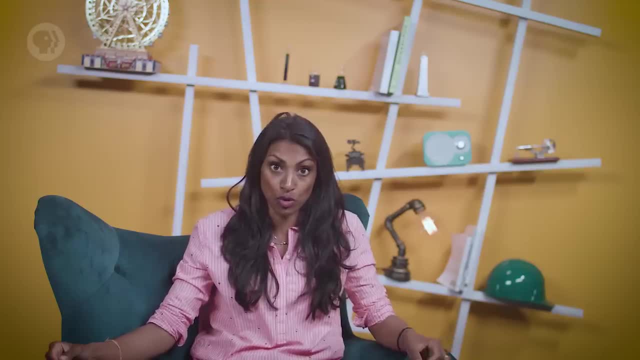 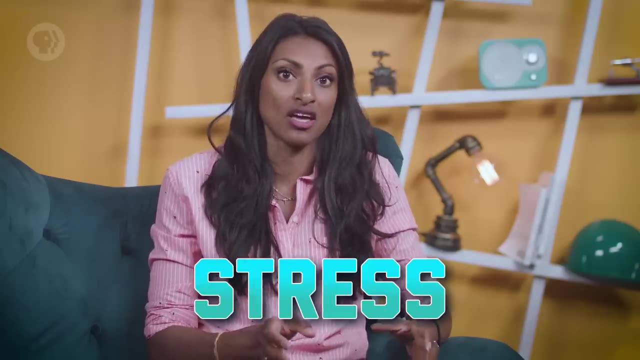 Because of this, the fluid particles in contact with the bottom plate will move with it, while the fluid particles at the top will stay in place with the stationary plate. This is all happening due to stress, the force that's applied to a cross-sectional area of an object or substance. 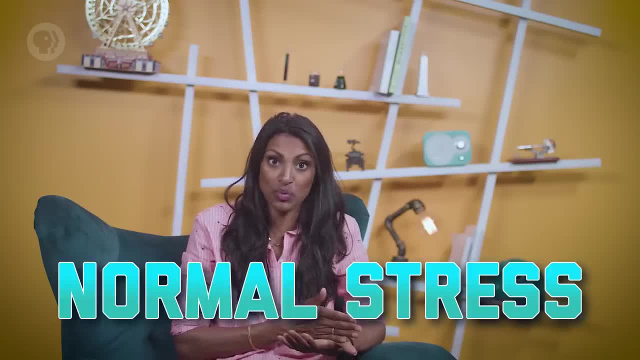 If the force is normal or perpendicular to the surface of the object, then we have normal stress. If it's parallel, then we have normal stress, Then we have shear stress. You thought I was gonna say parallel stress, didn't you? 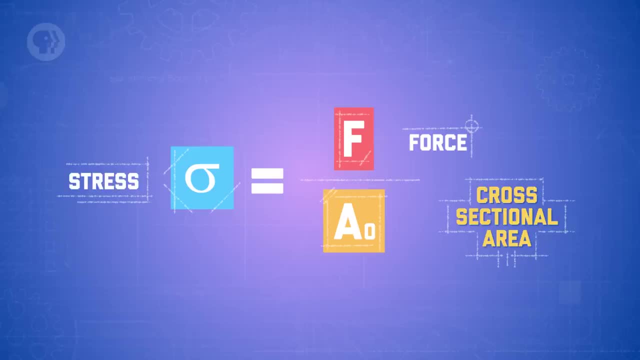 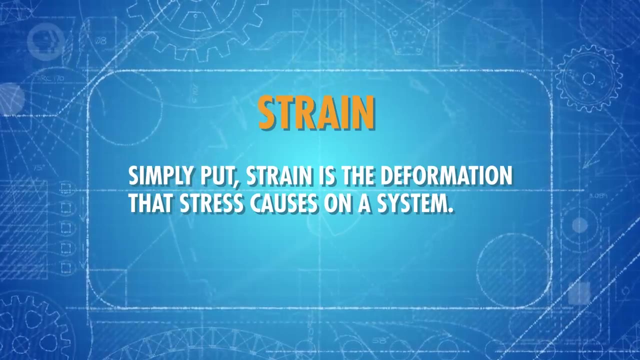 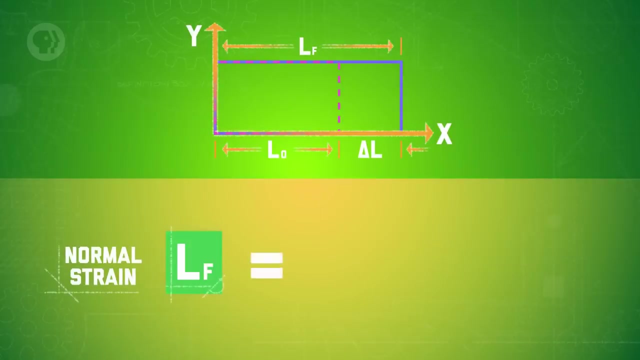 We can find stress by taking the applied force and dividing it by our cross-sectional area. Now, once a fluid is stressed, the degree to which it stretches is called strain. Simply put, strain is the deformation that stress causes on a system. If the deformation causes something in a system to become either shorter or longer, then we can find its strain by taking the change in length and dividing it by the initial length. 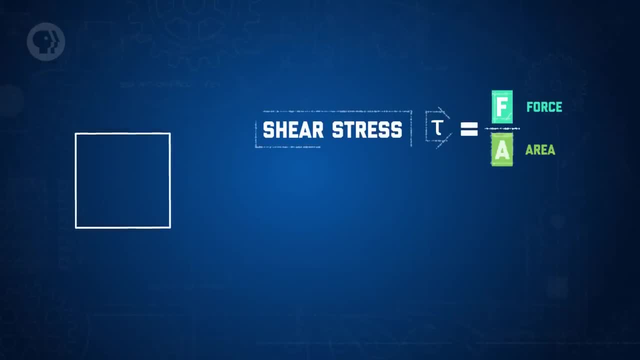 This is called normal strain. But if the deformation is a change in angle between two segments that had been perpendicular to each other, then we have shear strain, And we can find that by subtracting the change in angle from the original angle, which will 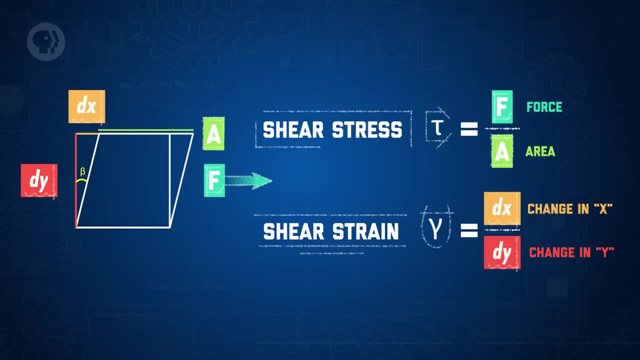 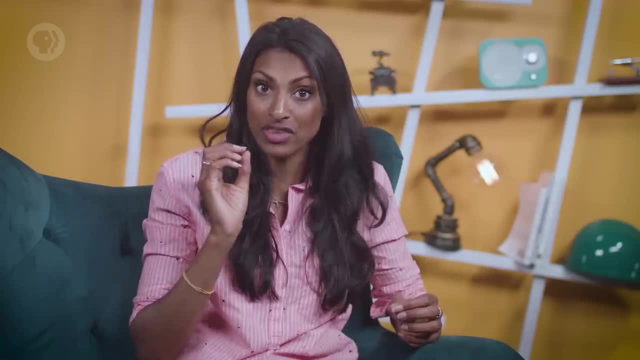 either be pi over 2 or 90 degrees, depending on your units. So all of this is what would happen if our bottom plate was moving. But what if neither plate moved and we had a pump driving the flow of the fluid between them? 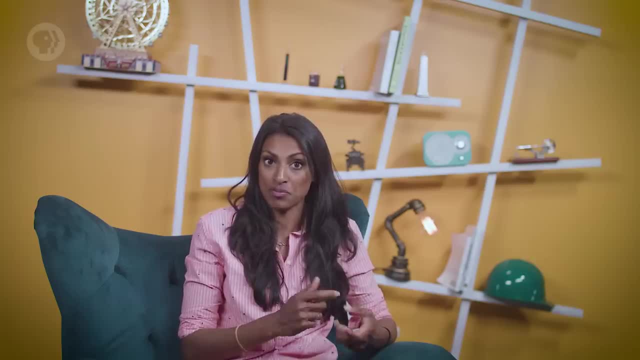 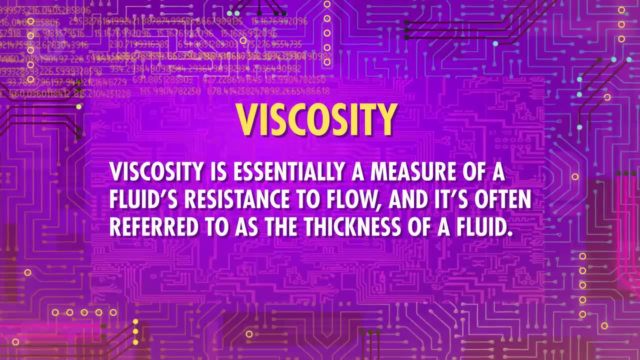 Well, the same no-slip condition would apply, so while the fluid moved, its particles at the surface of the two plates would stay stationary. But another thing we need to take into account is viscosity. Viscosity is essentially a measure of a fluid's resistance to flow and is often referred. 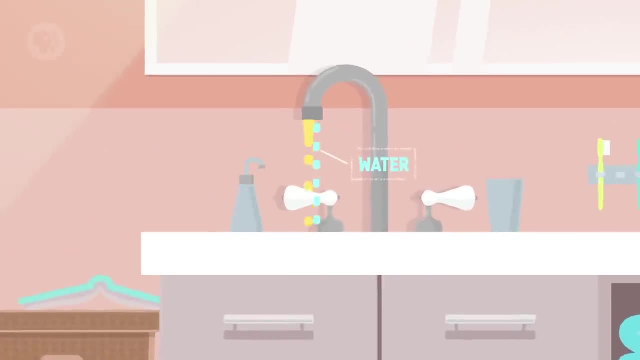 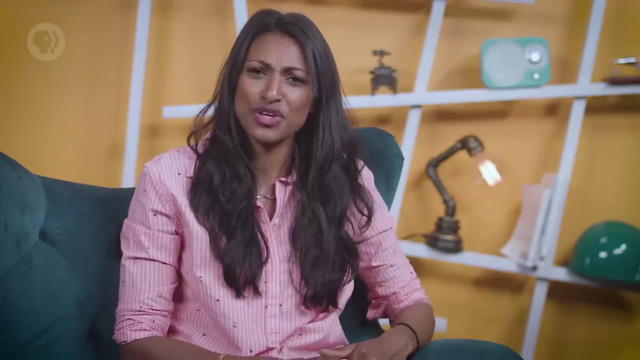 to as the thickness of a fluid. For example, water has a low viscosity since it flows pretty easily, while honey and other thick sticky fluids have a much higher viscosity. Some fluids will also thicken when exposed to stress, like when you whisk water mixed. 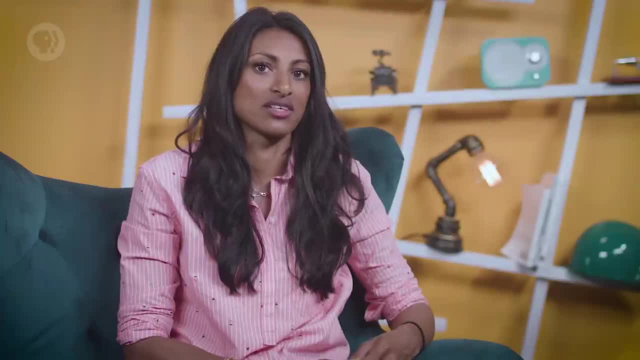 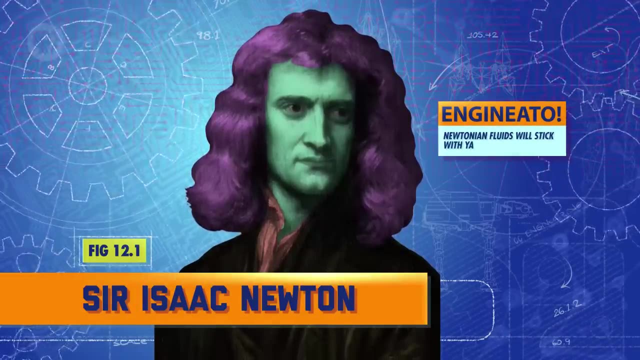 with cornstarch, But others will thin out when exposed to stress, like quicksand, which is just water mixed with lots of sand. The great Sir Isaac Newton gave us a way of describing how fluids move with his law, the law of viscosity. 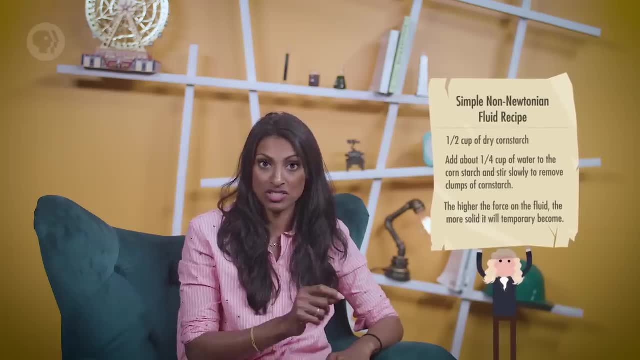 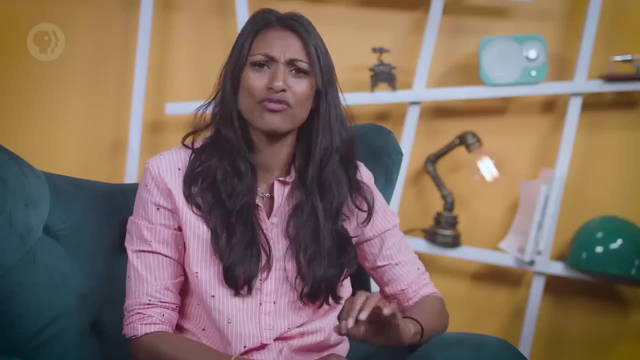 Simply put, this law describes Newtonian fluids as fluids with a viscosity that's independent of stress. No matter how much stress you put on the fluid, its viscosity never changes. While no real fluid is perfectly Newtonian, many fluids like air and water are close. 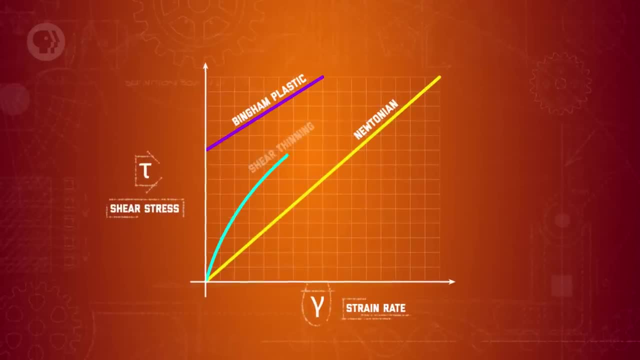 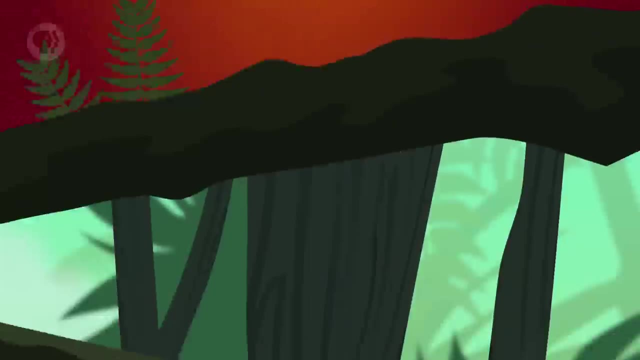 enough that we can think of them that way. Non-Newtonian fluids, on the other hand, don't follow the law of viscosity. Their viscosity can change under stress, and therefore their strain can too. A non-Newtonian fluid will actually thicken or thin out if you apply a force to it. 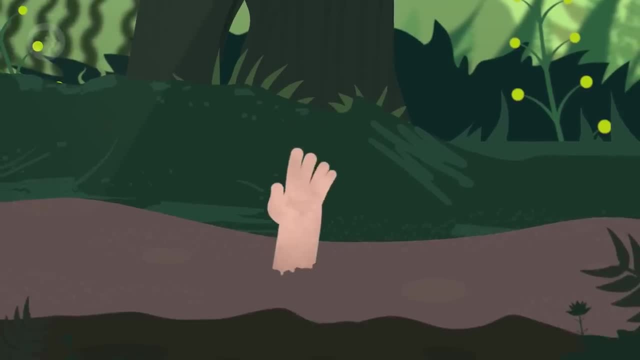 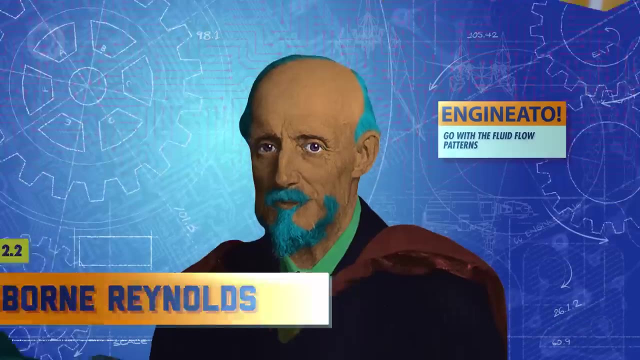 Which is exactly what happens when you step into quicksand. The stress of you stepping onto it makes it become less viscous, And then you're in trouble. Now there's still the matter of how one fluid moves within another fluid, And to understand that we should turn to the work of British engineer Osborne Reynolds. 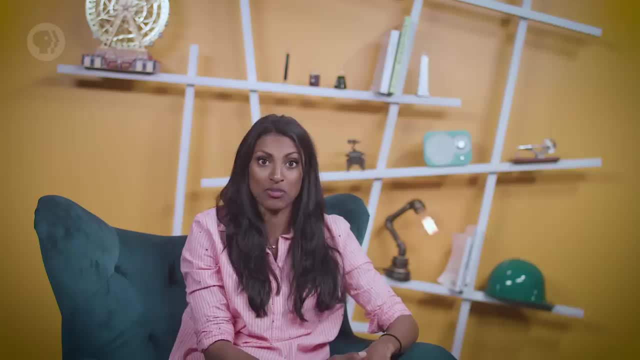 In 1868,, just a year after graduating from college, Reynolds became the first professor of engineering at Owens College in Manchester. He spent much of his career studying fluid mechanics and one of his greatest contributions was his work on fluid flow patterns. In 1883, Reynolds conducted an experiment 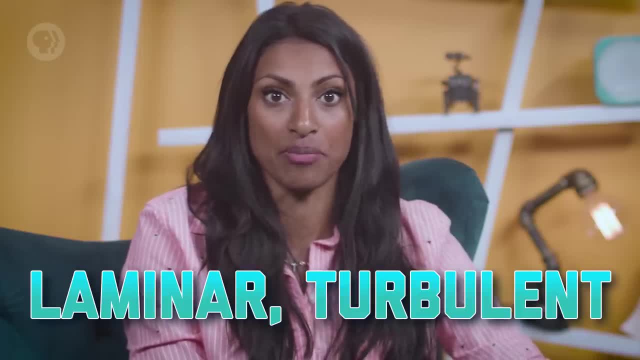 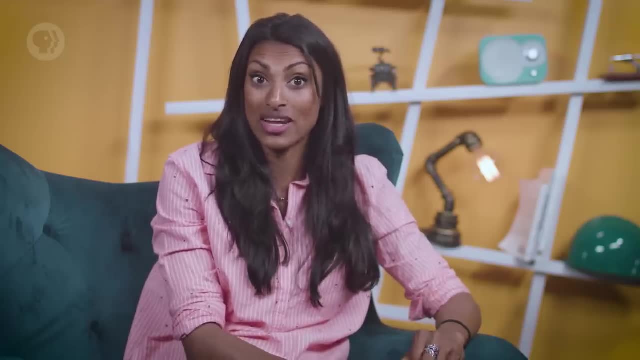 That revealed there are two main types of flow in a pipe – laminar and turbulent. This experiment was so influential that the device he used to conduct it was still used well into the 21st century. In his experiment, Reynolds used a colored fluid with the same density of water and injected 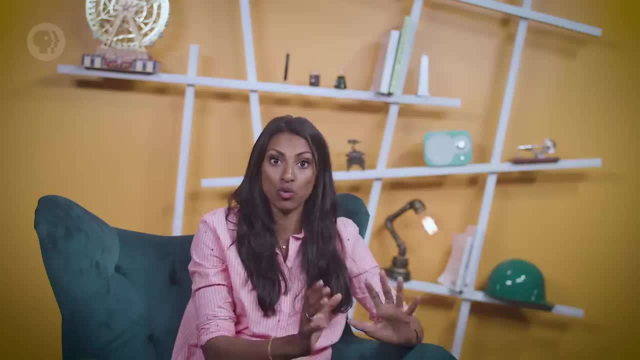 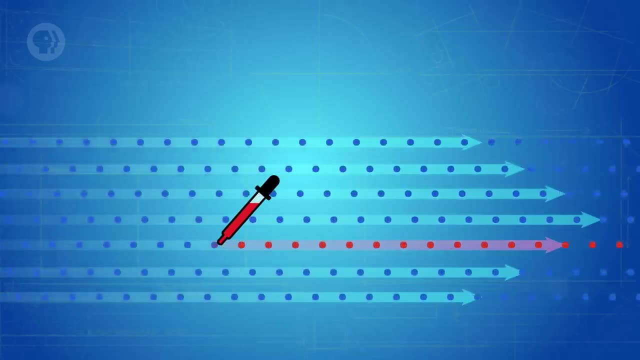 a very thin stream of it into a large transparent tube with water flowing through it. When he injected the dye into slow-moving water, the flow of the dye maintained its place and pattern in the center of the water. We call this laminar flow. 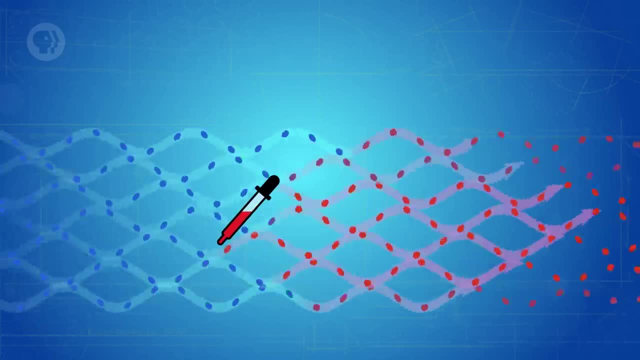 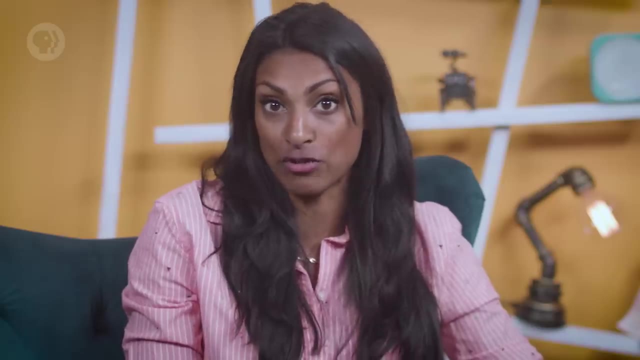 Once Reynolds injected the dye into water, that was moving fast. the dye spread out and diffused, mixing with water and coloring it. This is called turbulent flow. Those were the two main types of flow that Reynolds found, but we also have something called transitional flow. 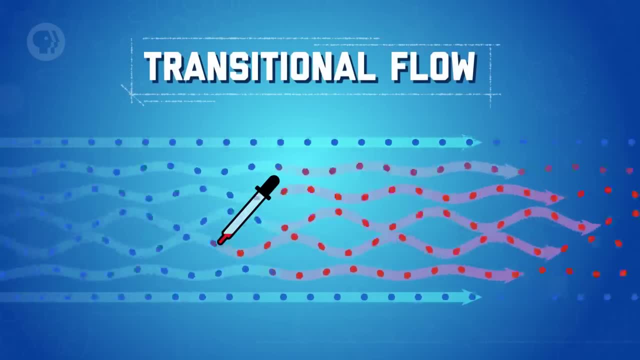 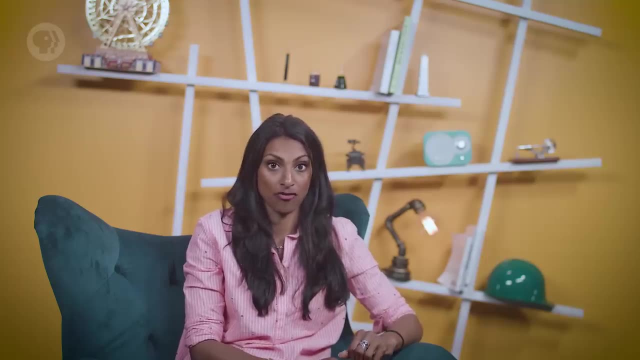 Transitional flow is a mixture of laminar and turbulent flow. It often has turbulence in the center of the pipe and laminar flow near the edges. Reynolds' experiment allowed him to determine when the transition would occur from laminar to turbulent, giving us the quantity we now know as the Reynolds number. 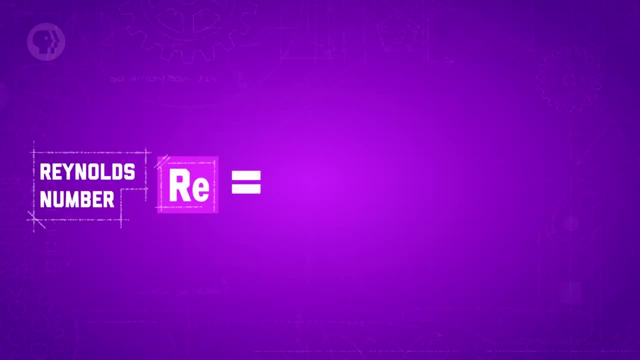 We can find Reynolds' number for the flow of a fluid in a pipe by taking the diameter of the pipe and multiplying it by the velocity of the fluid and the density of the fluid, then dividing all of that by the viscosity of the fluid. Now the value we get for our Reynolds number will be dimensionless, meaning there are no. 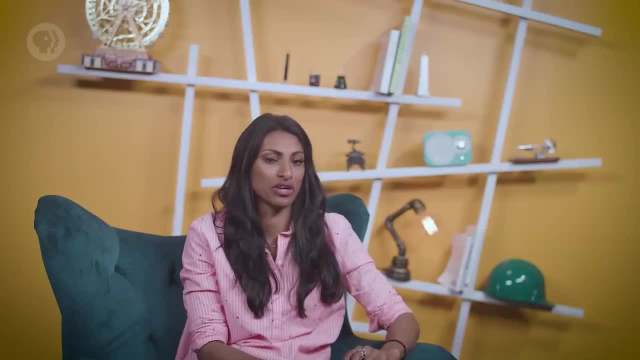 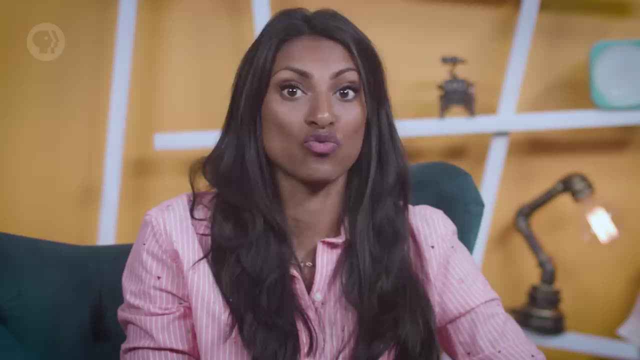 units attached to it. But it can tell us a lot about the movement of a fluid. It lets us know how predictable or chaotic our fluid flow will be. That's because we can look at the Reynolds number as a ratio of inertial forces to viscous forces. 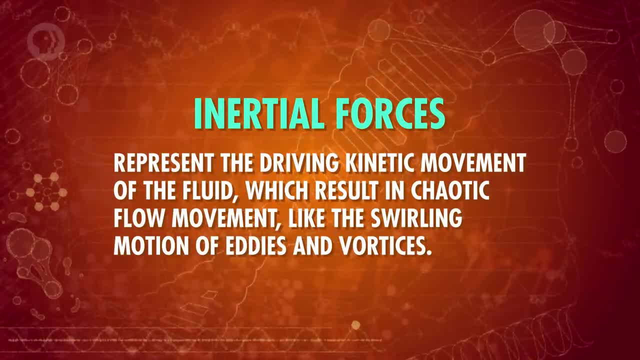 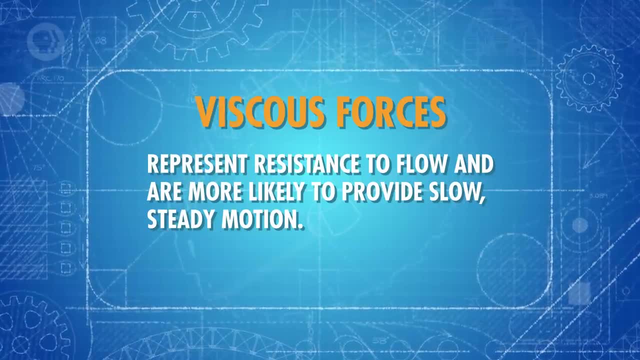 Inertial forces represent the driving kinetic movement of the fluid, which result in chaotic flow movement like the swirling motion of eddies and vortices. Viscous forces represent resistance to flow and are more likely to provide slow, steady motion. 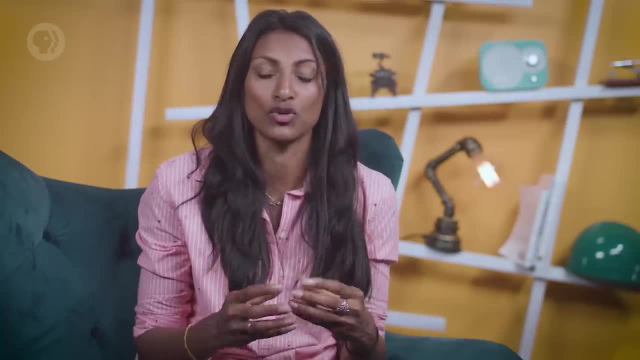 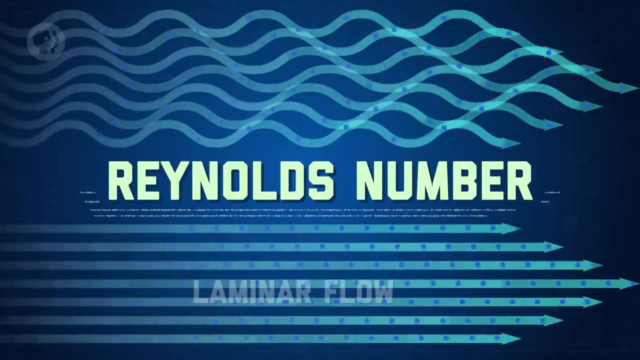 So the more powerful your viscous forces are, the slower and more controlled the fluid's motion will be. The higher your inertial forces are, the more chaotic your flow will be. Therefore, a low Reynolds number represents laminar flow, while a high Reynolds number 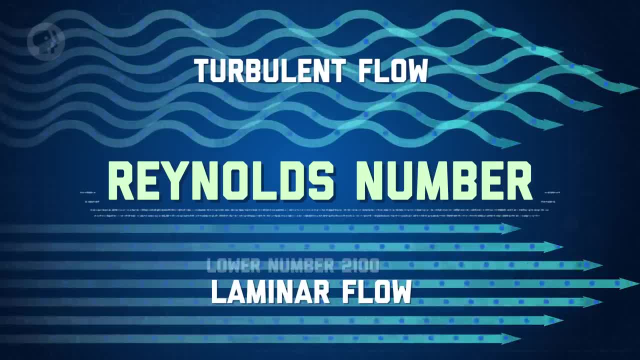 represents turbulent flow. In a pipe, laminar flows will use the momentum of the fluid. Fluid flows will usually have a Reynolds number lower than 2,100,, while turbulent flows will usually be higher than 4,000.. And a Reynolds number between these two values typically represents transitional flow.